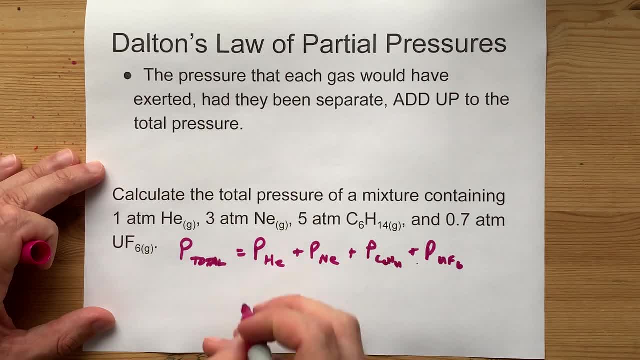 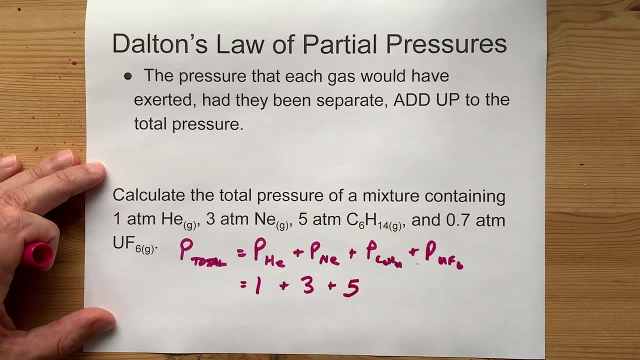 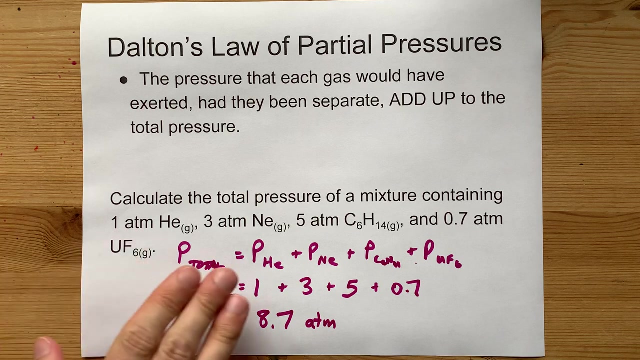 few as you want, but the total is the sum of each separately: One atmosphere of helium and three of neon, and five of hexane and 0.7 of uranium hexafluoride- it doesn't matter what they are- gives you the total pressure of the mixture of those four things Now. so this is 8.7. 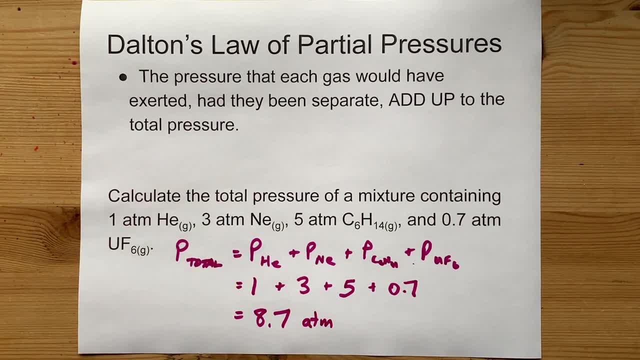 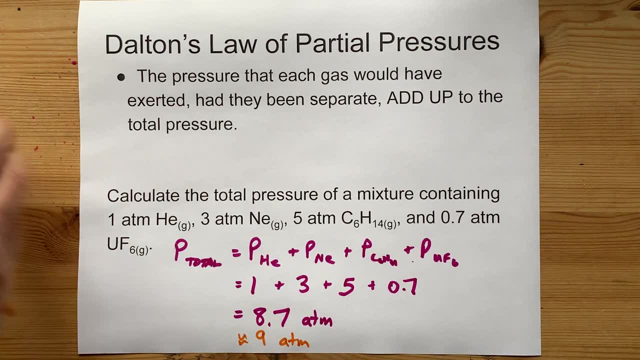 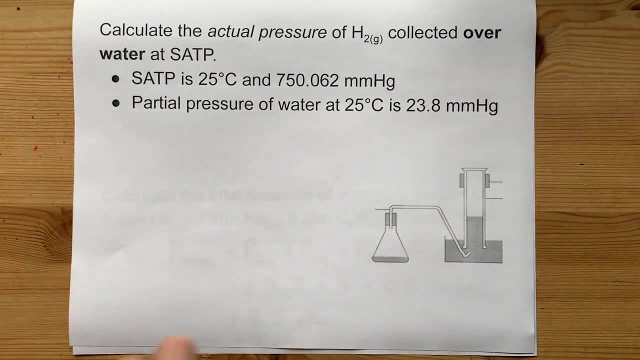 atmospheres because we're adding and there's no decimal places here. If you're gonna use sig figs you're gonna have to say 7 atm, but that's neither here nor there. The classic application of Dalton law is when you're collecting gas over water. what we mean is that if there's a 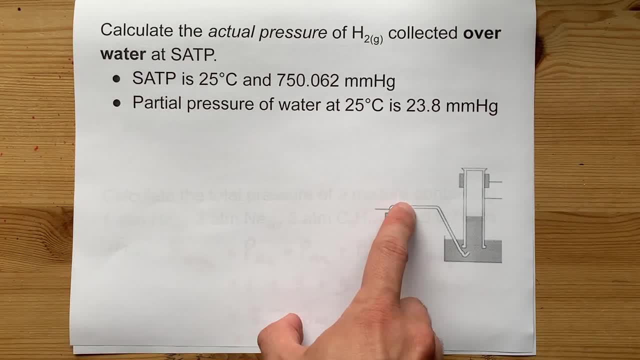 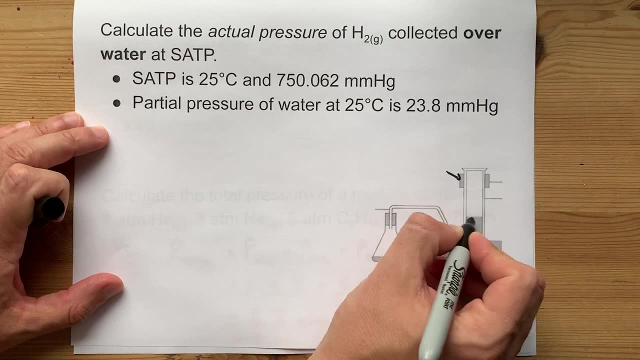 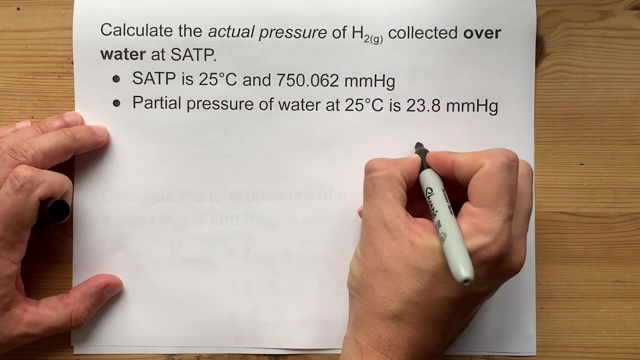 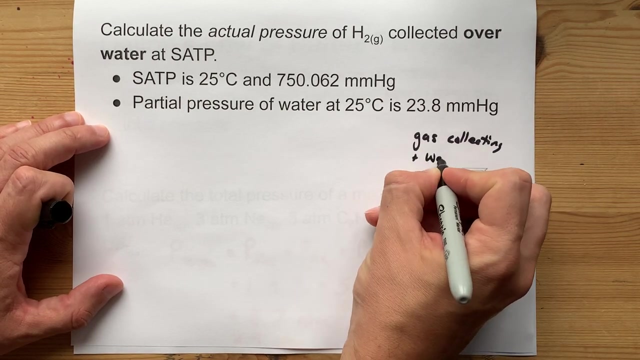 chemical reaction that's creating gas here and you bubble it through a tube into water. the gas itself is going to collect here and displace the water like push the level of water down, but what's up here is the gas that you're actually collecting a little bit of water, because liquid water has a vapor pressure and some of those water molecules. 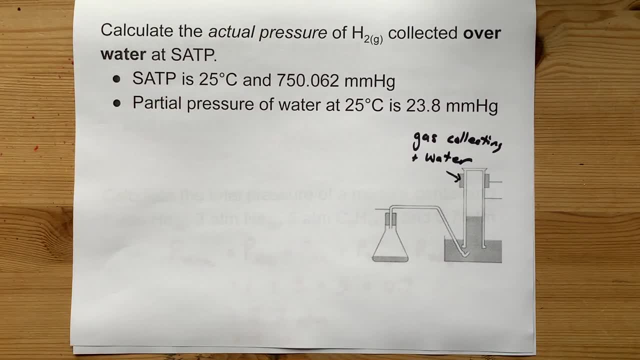 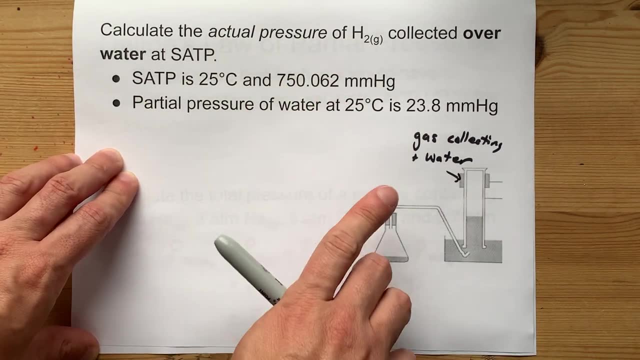 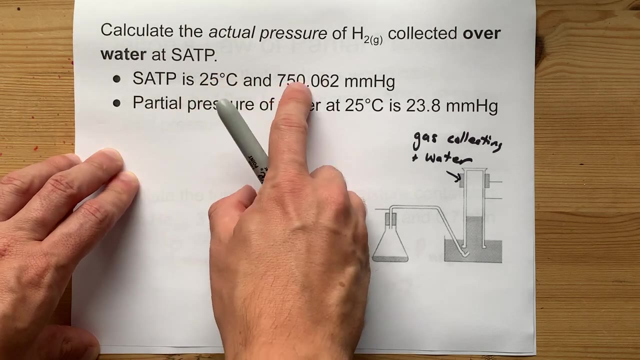 are going to have evaporated into the gas phase, So the actual pressure of the gas you're collecting is never the same as the ambient pressure. Now we're going to say this is at ASTP, which is 25 degrees Celsius and 750-ish millimeters of mercury. That's just the unit I chose to use here. 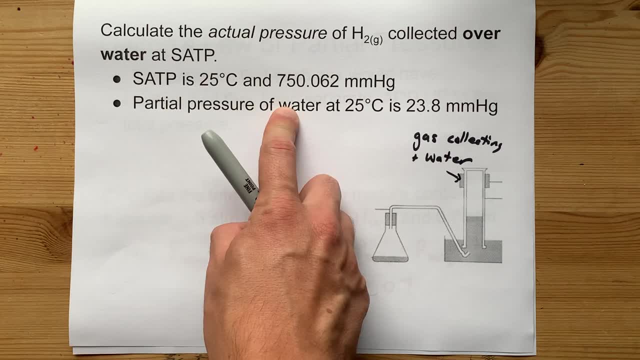 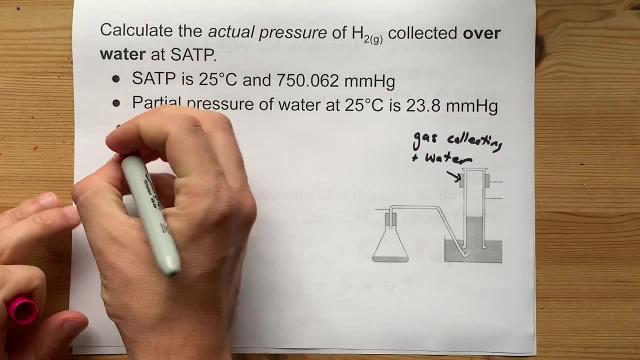 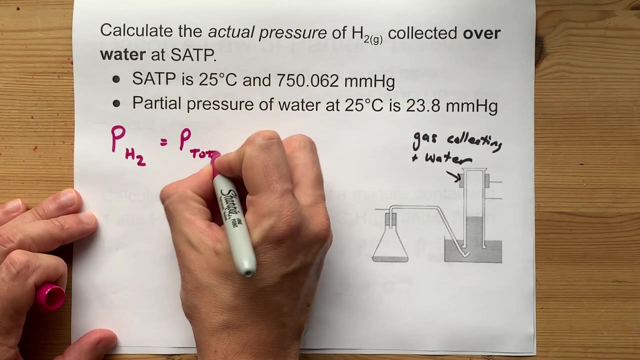 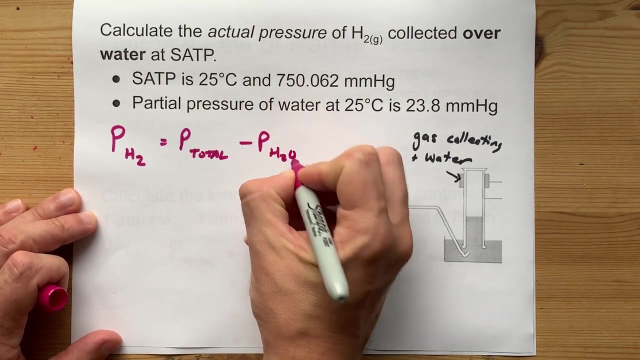 But at 25 degrees Celsius water provides 23.8 millimeters of mercury of pressure on its own, So the pressure of the actual hydrogen you're collecting is less than 750.. 750 millimeters of mercury is the total pressure, but you have to take away the contribution of water to that. 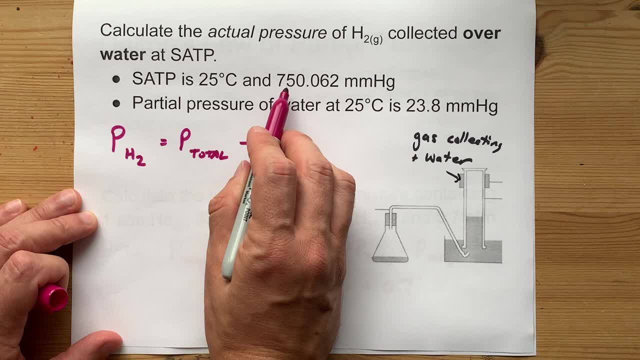 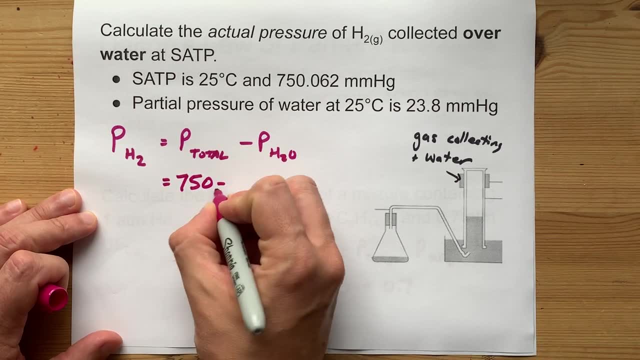 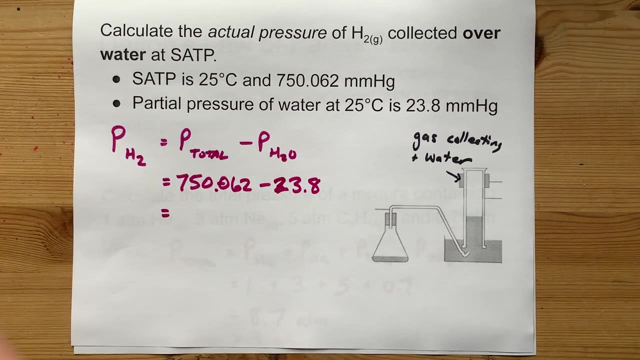 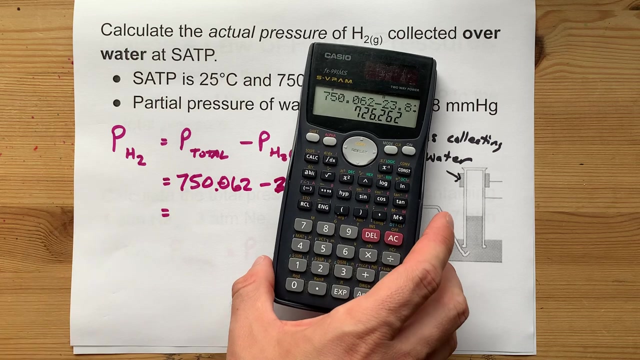 This space in here is at 750.. 750, but 24 of it is just water. So 750.062 minus 23.8.. I'm going to have to do that on a calculator: 750.062 minus 23.8. I get 726.262. 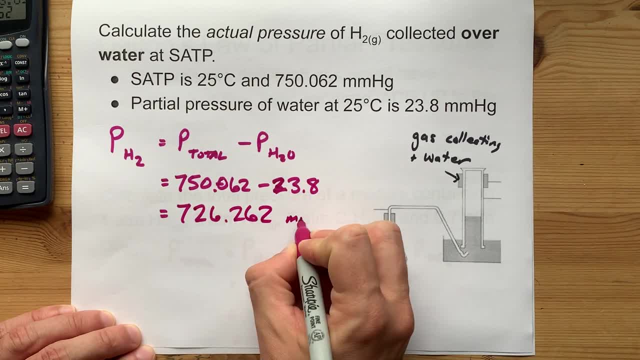 So 750.062 minus 23.8.. I get 726.262.. So 750.062 minus 23.8.. I get 726.262.. So 750.062 minus 23.8.. I get 726.262.. 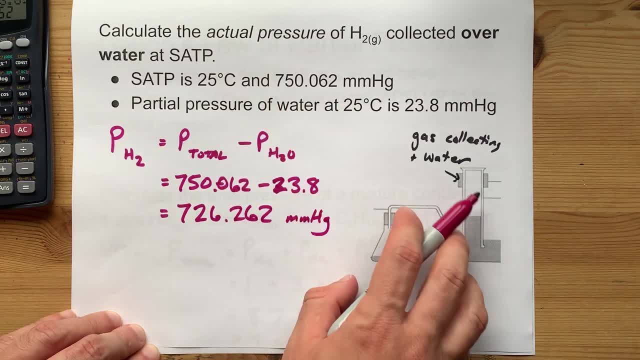 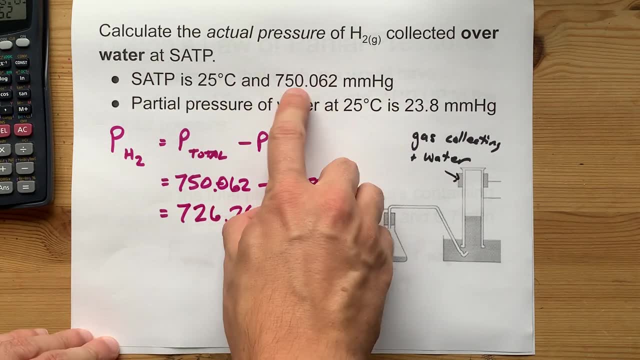 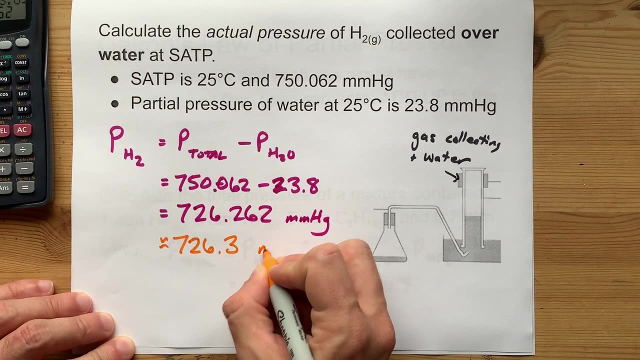 That's significantly less than the total pressure that you might have thought hydrogen was providing. there And again, with the sig figs, we've got three decimal places here and one here, So we're going to have to round this to 726.3 mmHg. 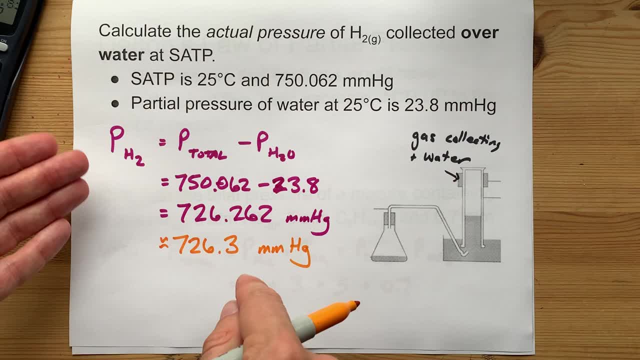 If you're asked for the number of moles of hydrogen that were produced, you're using this pressure, not 750. That is water plus hydrogen, So you get 726.3 mmHg. Another classic is being given the total pressure. 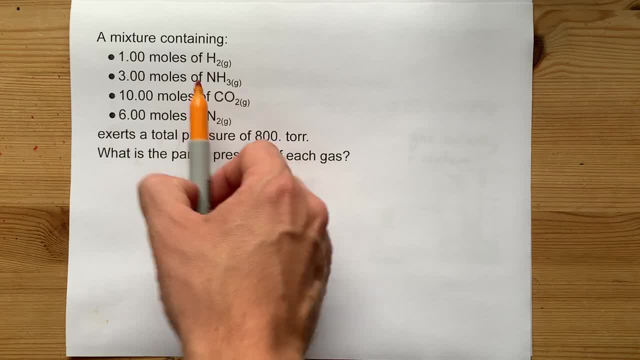 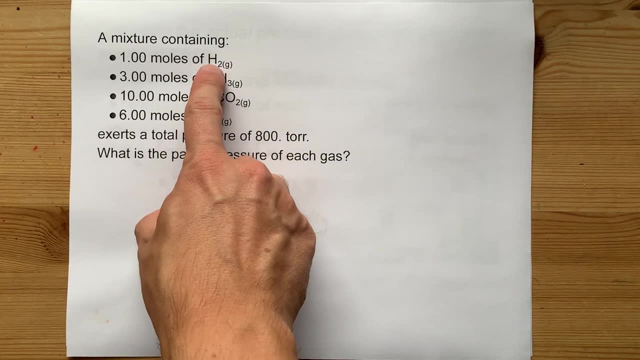 And the numbers of moles of each of the components. Now, this one's perhaps a little bit tricky, But what really matters is that it doesn't matter what the identity of each of these are. This in total is 20 moles. 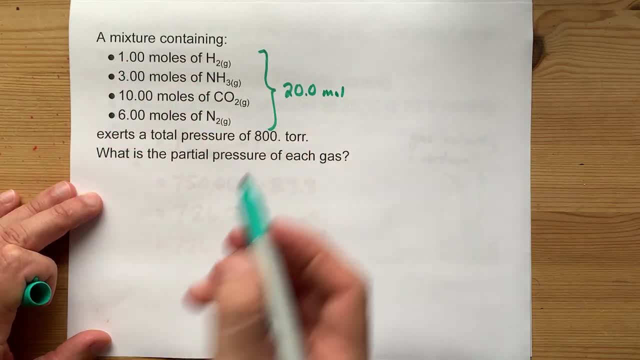 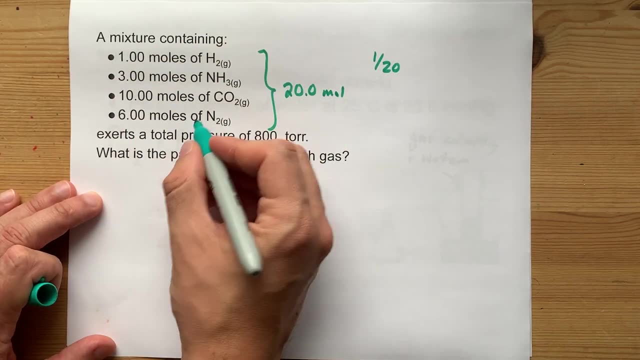 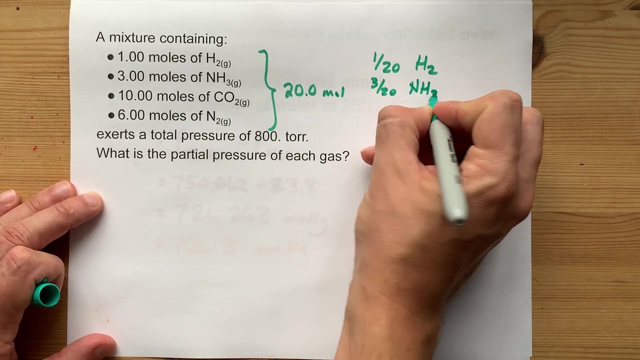 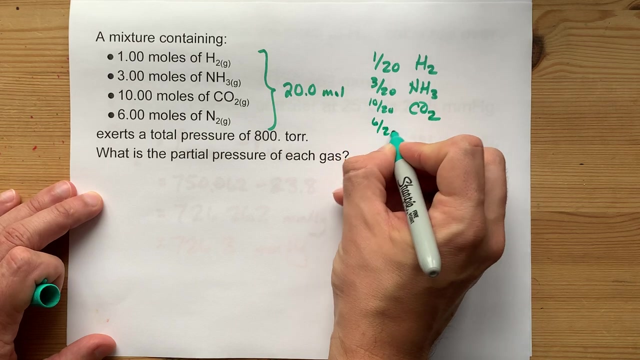 I got that by adding these together: 120 of these: 1 20th of the whole. 1 20th of all the molecules here are hydrogen. 3 20ths of all the molecules are ammonia, 10 20ths or one half of all the molecules are carbon dioxide and 6 20ths. 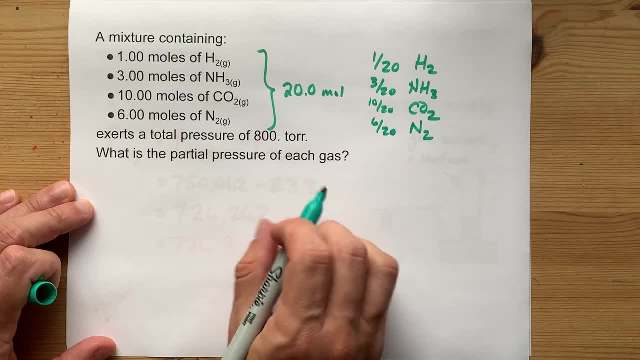 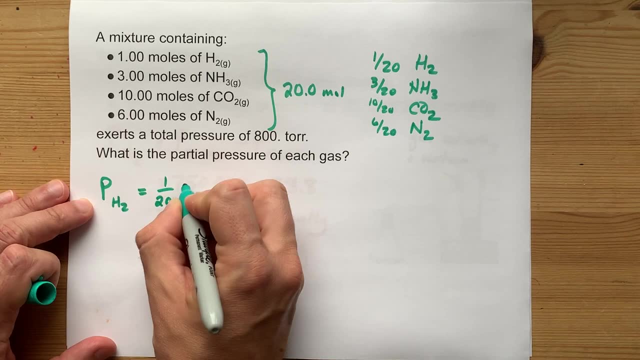 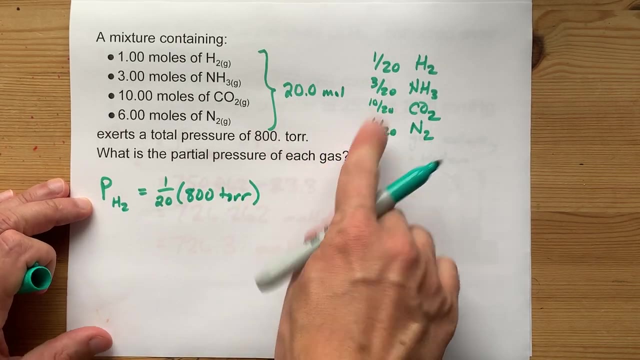 are nitrogen. If you're given the total pressure, you can calculate the pressure of the hydrogen gas knowing that it is 1- 20th of the total pressure. This 1 20th, 3 20ths, 10 20ths, 6 20ths are called. 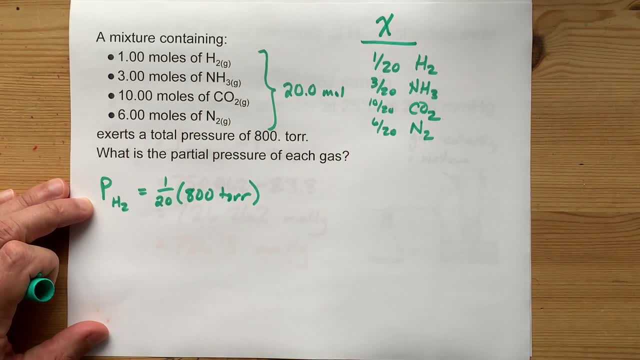 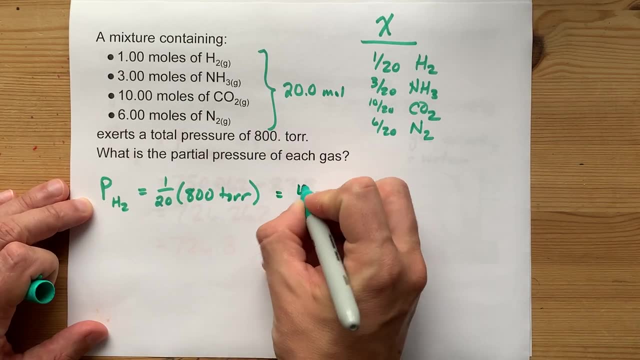 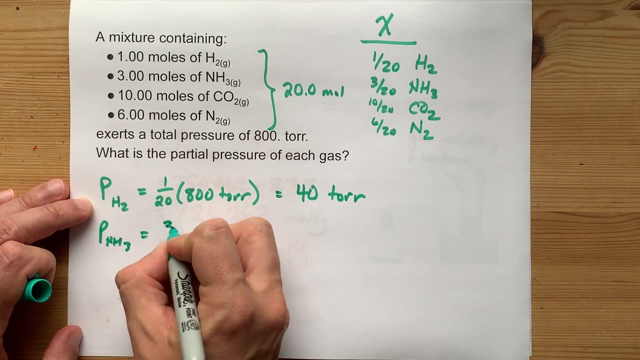 the mole fractions of each of those. But again, each of those is the fraction of the contribution to the total pressure, So that means we have 40 torrs of hydrogen. The pressure of ammonia is 3, 20ths of the total pressure, So that means we have 40 torrs of hydrogen. 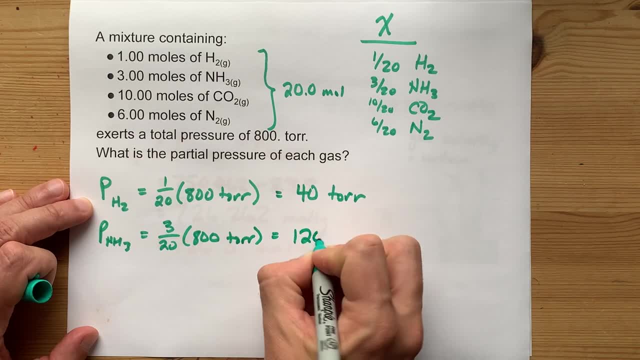 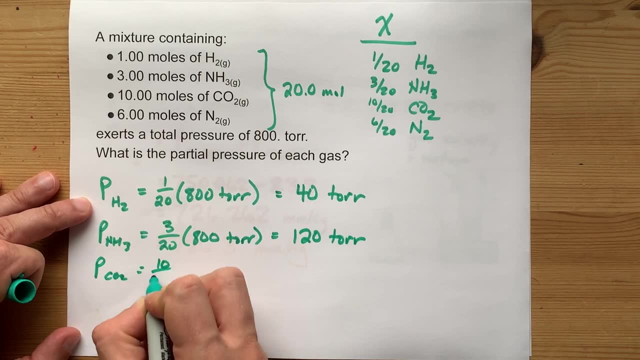 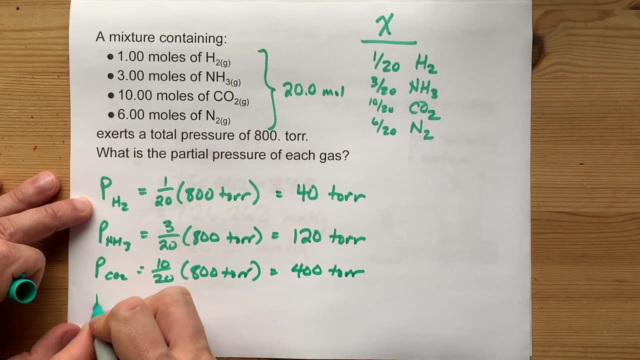 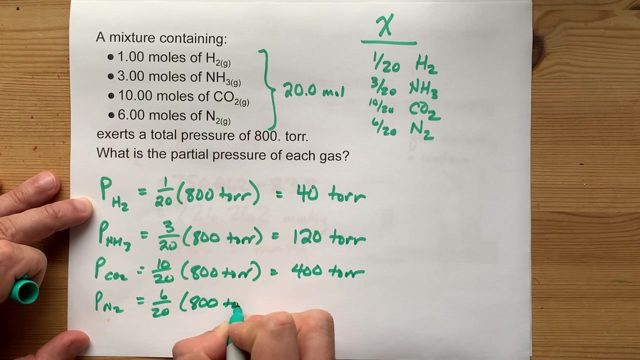 Of 800,, which means it was 120 torr. The pressure of carbon dioxide is half of 800,, which is 400 torr, And the pressure contributed by nitrogen would have been 6 20ths of 800,, which is 240 torr. 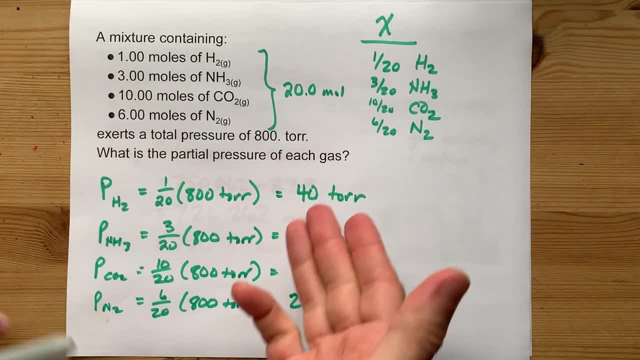 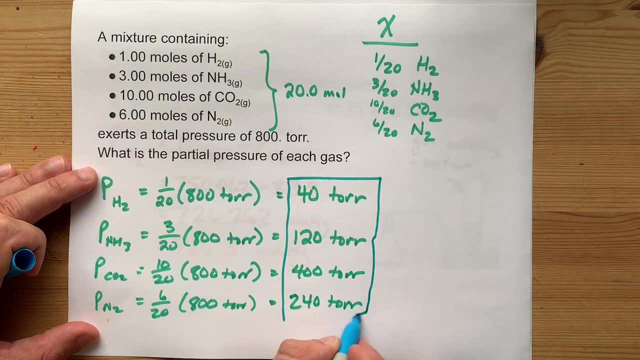 The reason I didn't just skip all that and wanted to actually do the calculation is that the sum of each of the partial pressures together, when you add them up, should be the total pressure. Dalton's law of partial pressure says the total pressure is the sum. 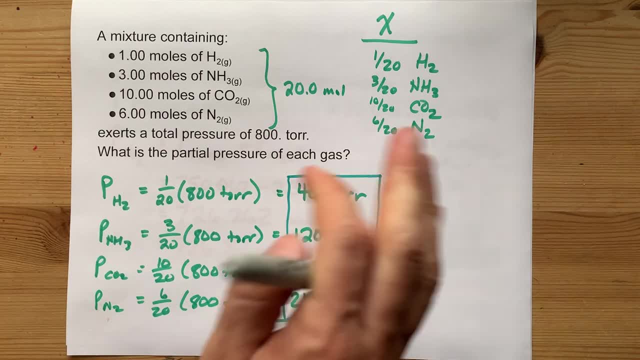 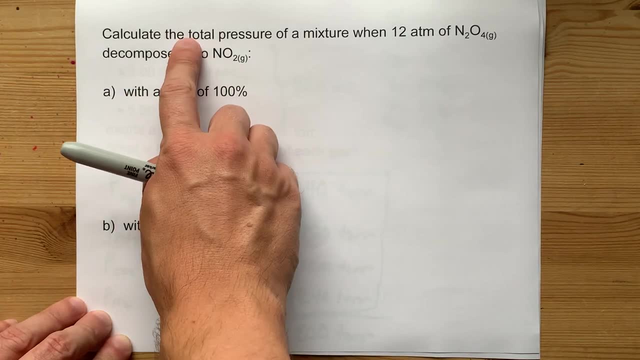 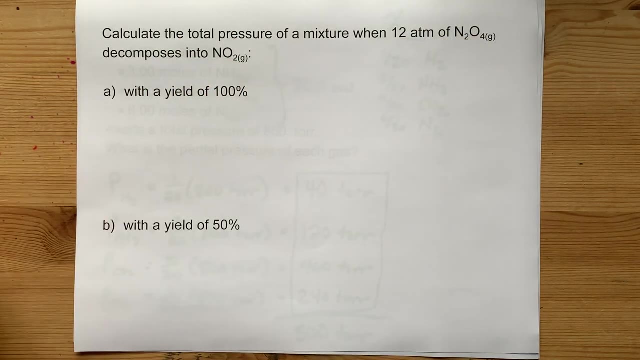 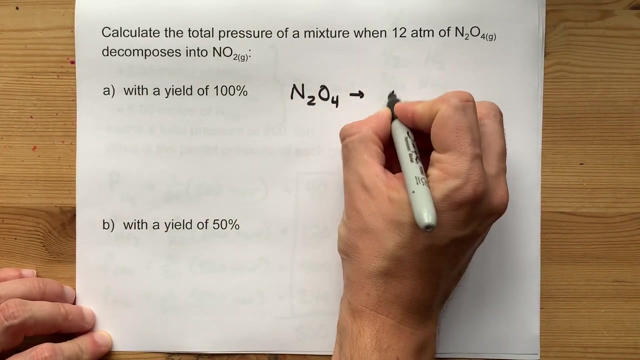 of the partial pressures of each component. Beautiful, I've got a challenge question up here. I want to know the total pressure of a mixture when 12 atmospheres of N2O4 decomposes into NO2.. Let's do the chemical reaction for that first: N2O4 breaking apart to make NO2.. 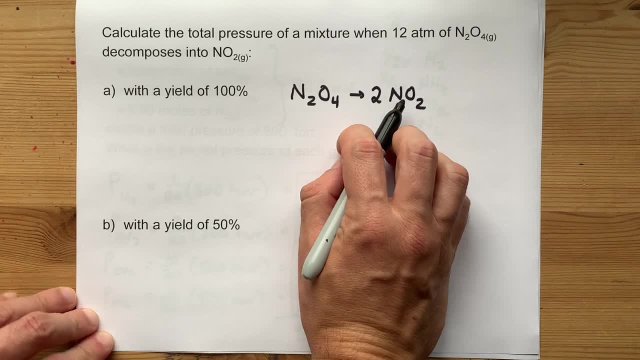 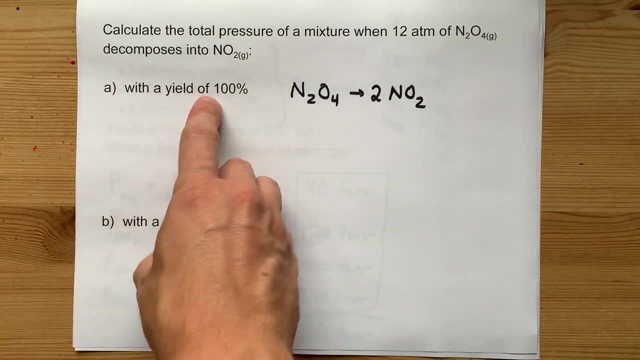 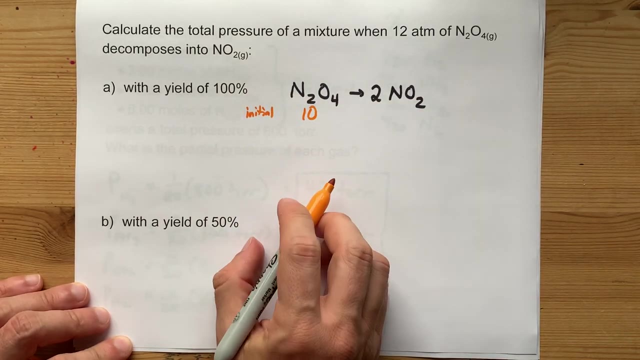 To balance this, I need to note that I get two NO2s for every N2O4.. Now part A that I've rigged is the yield of 100%. So we are going to start out with 10 atmospheres of N2O4, but we are going. 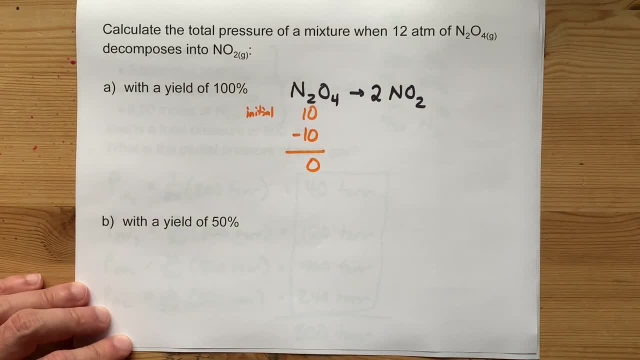 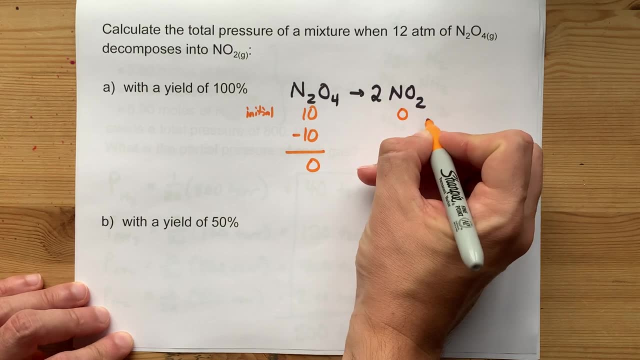 to use up all of it so that there is none left. That's what it means to yield 100%. No reactant left. The NO2 starts out at zero, but we get two of them for every one of those that broke apart. 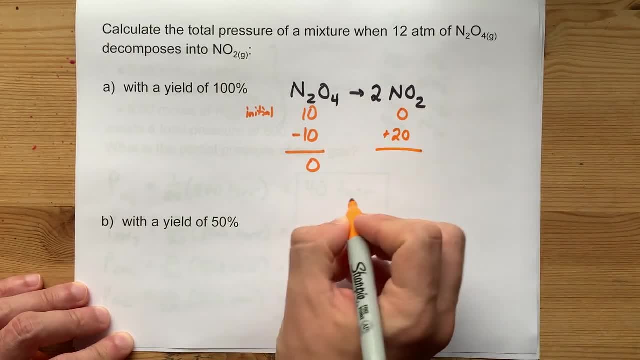 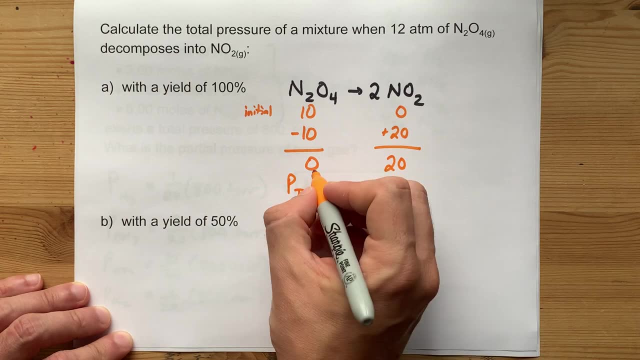 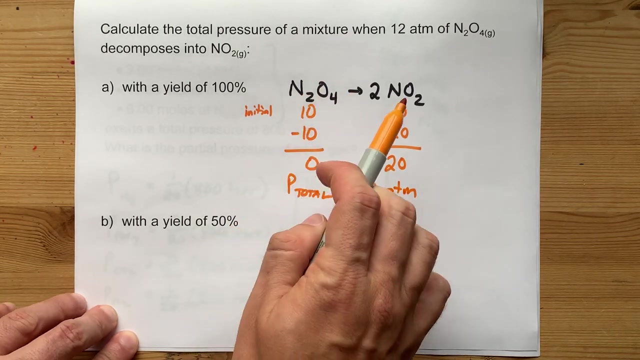 That means we're going to gain 20 atmospheres of NO2.. The total pressure here is the sum of these two, but actually there isn't any of that. The total pressure is 20 atmospheres. That should make sense because it's a one for two exchange of.